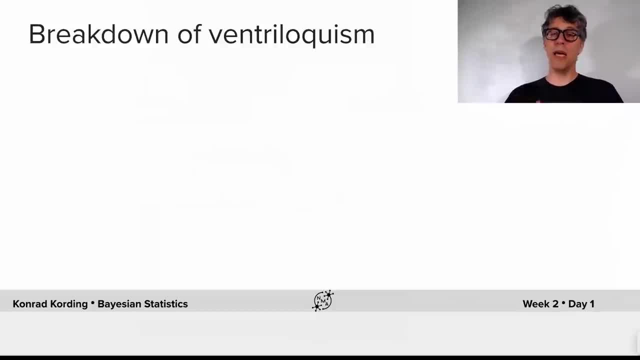 We can try and give you an example of that. So what we'll do now we will put all the sound onto the left side, where really my face is on the right side, And now we will put all the sound back on the right side. If you have the right setup, you will have seen that in the first case. 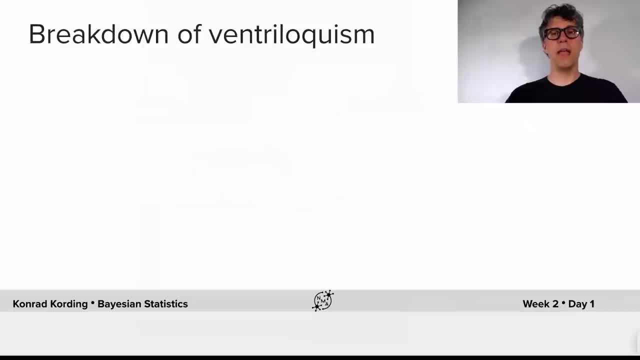 when the sound comes from the left and you see my face on the right and you're close enough to the screen, you will see a breakdown of ventriloquism So it doesn't sound anymore as if the sound is coming out of my mouth. 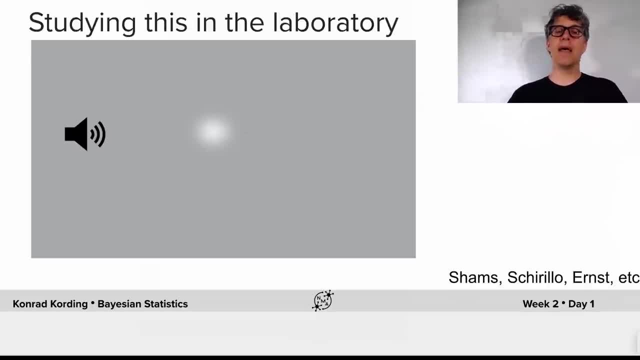 So we can study that in the laboratory just like before. So what's the difference? Well, it turns out that the only difference is that in standard experiments in that field, we look at two things that are very compatible: We have a visual stimulus somewhere here and a sound. that's 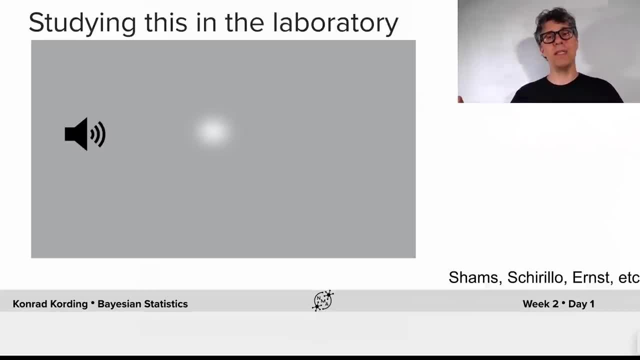 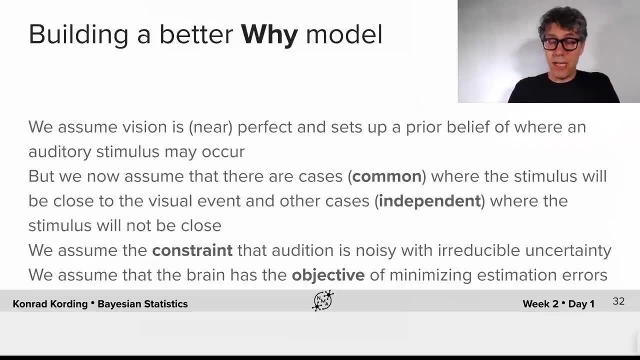 somewhere close by. If we make that difference very large, we get into a different domain. And now we will build a Bayesian model for this case Now, like we want a model that now also can describe the phenomenon that if we make two things very 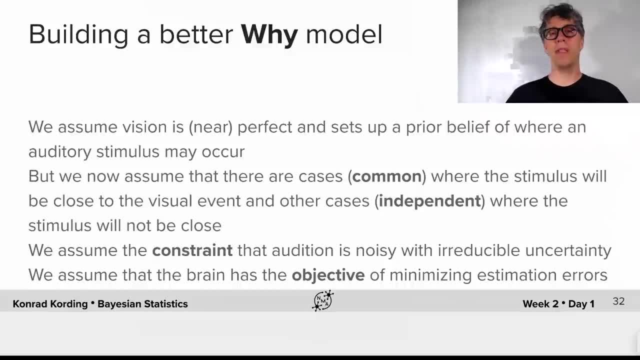 different from one another, that they break apart, that they're processed independently. So we will build another Bayesian wire model. So we again assume that vision is near perfect and sets up a prior belief of where the auditory stimulus may occur. But we now assume that it's. 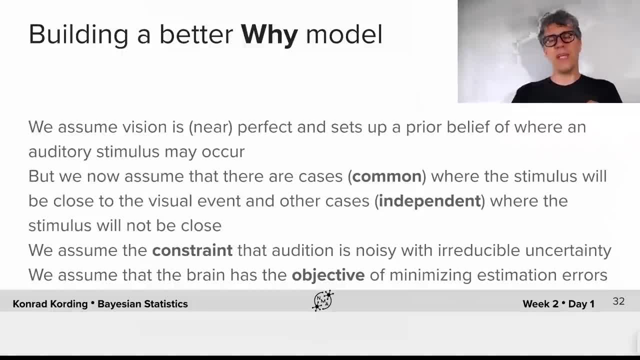 not the case that in all cases we expect the auditory stimulus to be close to the visual one, But we assume that it's not the case that we expect the auditory stimulus to be close to the visual one. So we assume that there's two implied cases. There's the common case, where the assumption is: 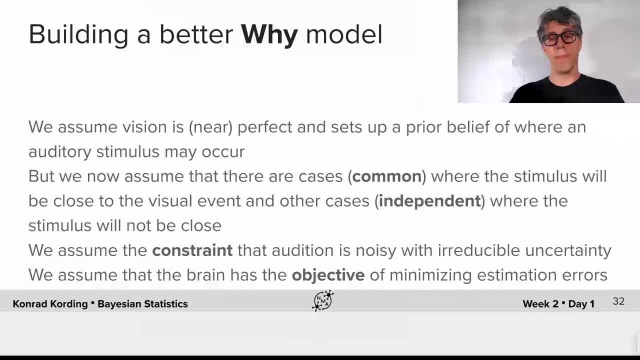 that the visual stimulus must be very close to the auditory one. And then there's an alternative case, the independent case, where we don't believe the two of them to be very close to one another. If anything, we allow the auditory stimulus to be very far away from the other one, And we again 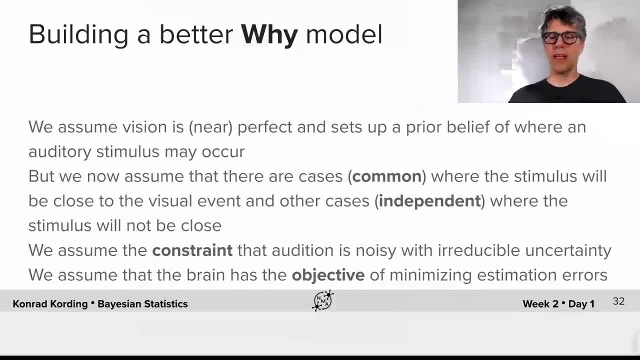 assume that audition has the constraint of having irreducible uncertainty. And we assume again that the auditory stimulus must be very close to the auditory one. And we again assume that the auditory stimulus must be very close to the auditory one. And we again assume that the auditory stimulus must be very close to the templ simulated. 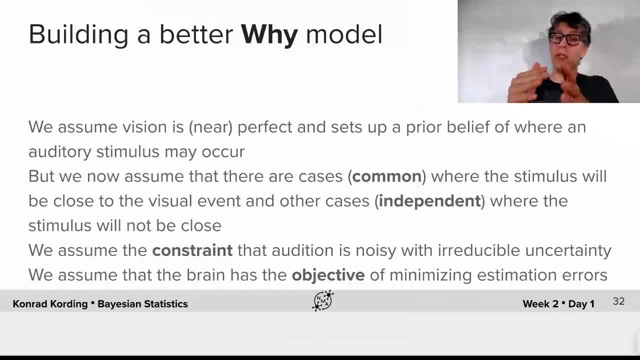 But what you see is like it's almost the same model. It's just we take one part where we did a strong simplifying assumption that the two things always belong together. It's just we take one part where we did a strong simplifying assumption that the two things always belong together. 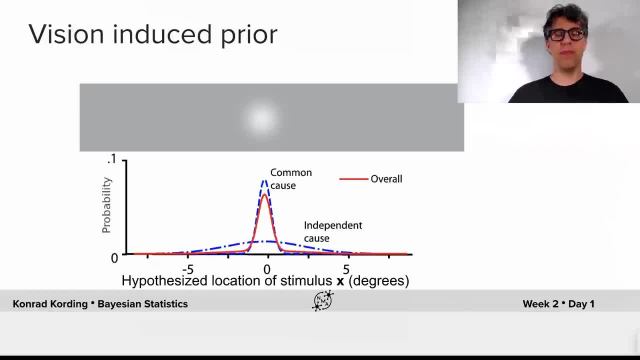 And now we relax that assumption. So What do we assume now? we assume that the vision in use prior isn't just a Gaussian, But it contains two parts: The common cause part, which is the Gautius we had it before, which is believe that the auditory stimulus often should be coming from close to where the 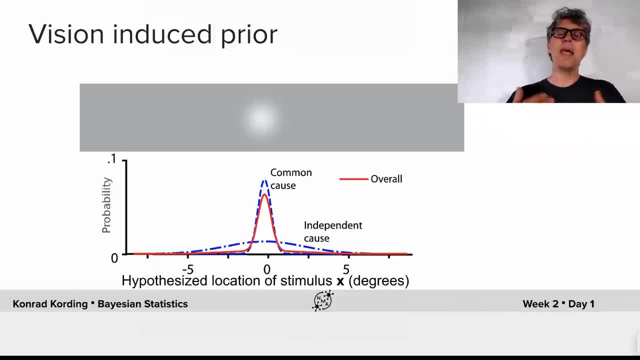 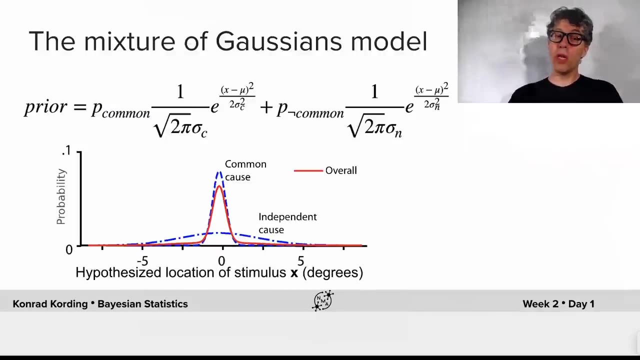 visual stimulus is. But then we assume a largely independent case where we might believe that they're somewhere close to one another, but it can be quite far away. So that's the so-called independent case. Now, how should we model this mathematic here? Well, we can say we want to have a mixture of Gaussians model. 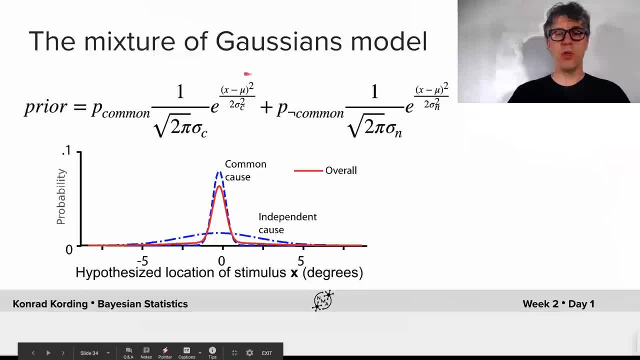 where we have one Gaussian that describes what happens when they're close to one another. Now here the standard deviation will be small. This is this narrow standard deviation and here that not common case- are the independent case where the standard deviation will be very large. We might. 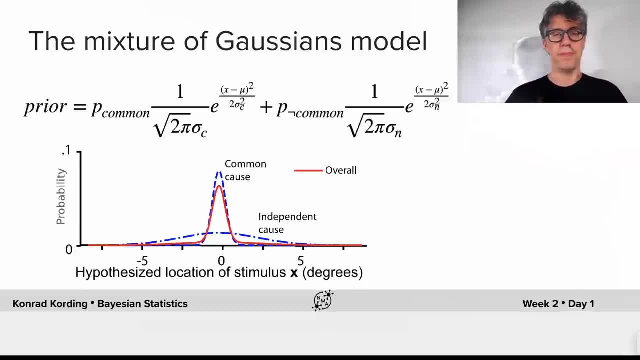 even want to believe that it's arbitrarily large. So this is the model. It implicitly assumes that the 、 that is set up by vision can have two very different cases. Either it belongs together and there's a common cause, and therefore the prior is narrow, or otherwise it's wide. 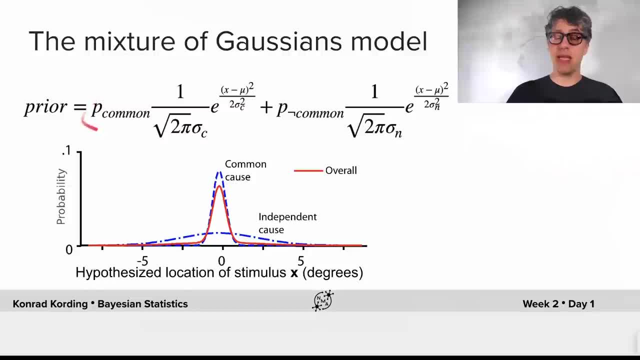 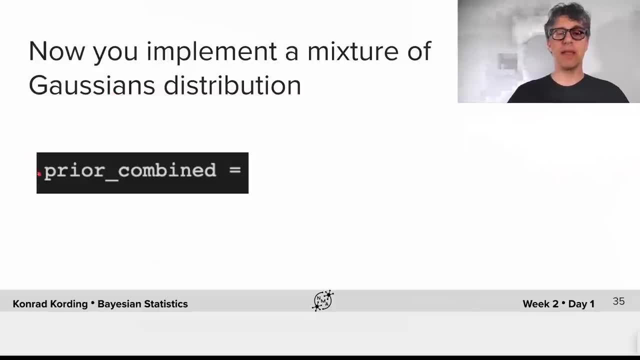 And both of them are possible. And you see, we have a parameter here, p common, that tells us how important one of them is relative to the other. Now it's time for you to implement that. Calculate the combined prior that has both components.